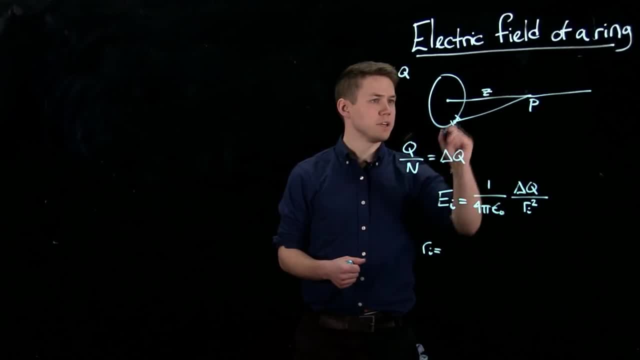 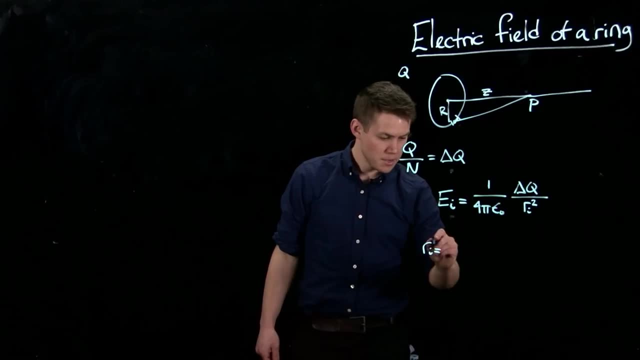 to give some labels. To be consistent with the book, I'll label this to be R- sorry, this to be Z- and this distance. so the radius of the ring is going to be capital R. So that means that Ri squared is equal to Z squared plus R squared. 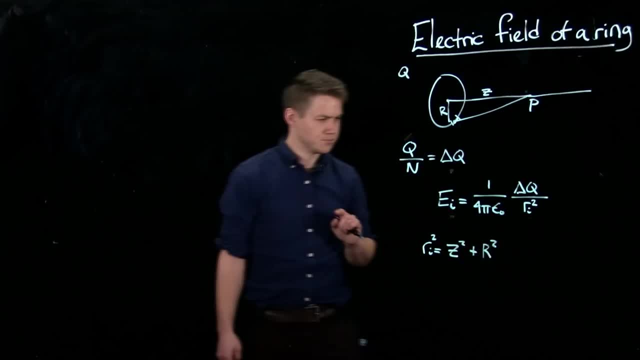 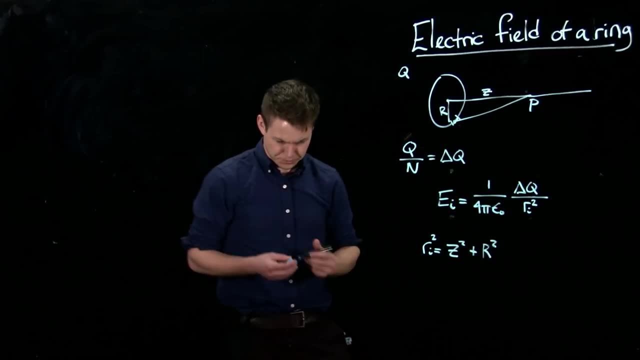 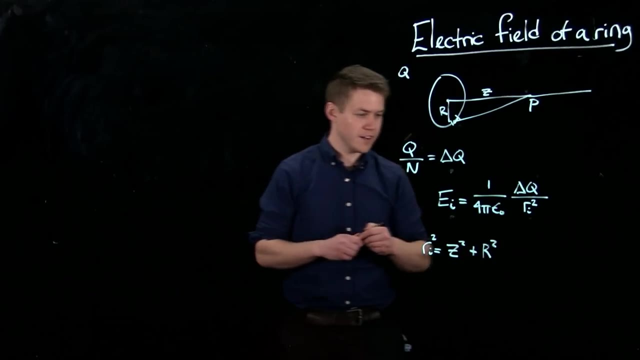 Okay, so I could plug that in right there. And so what else do I need? Well, I need to know- sorry, this delta Q, I already know from this term here, but there's one thing which is missing, which is that I have written down here a vector equation. So this: 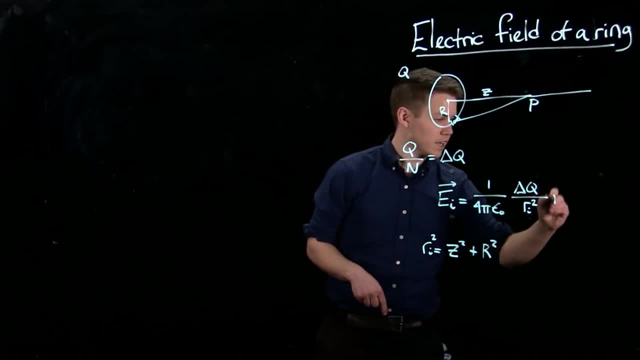 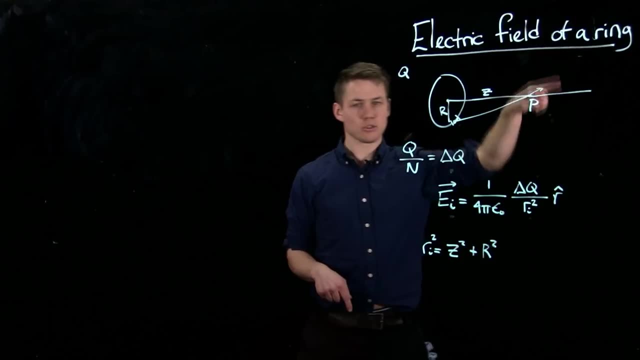 should have a vector equation on it and this should have an R hat. So this here would be really the electric field along a little vector pointing out of this plane. Now, what you can probably see already is that if this is the Z-axis, 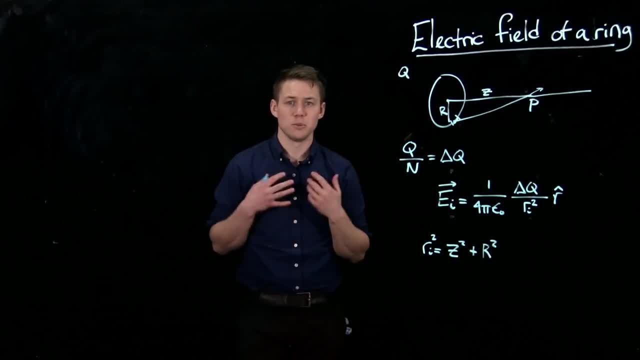 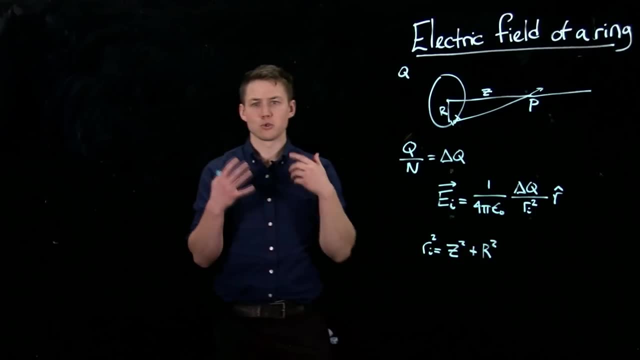 then the electric field along X and Y are going to be Z squared and then the Y-axis is going to be zero at P. And that's because there'll be a similar little vector pointing down from this point up here, and those will cancel out the Y. 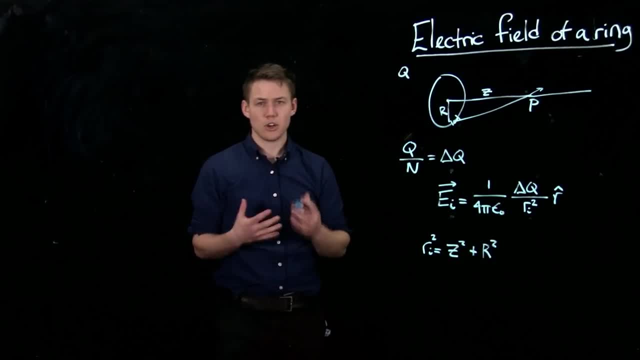 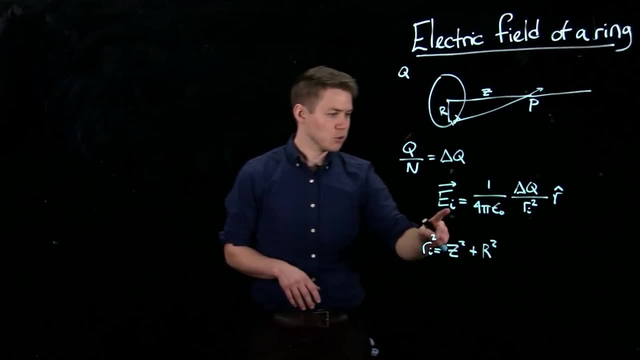 components if this is the Y-axis, And similarly, the same thing will happen for X. So the only part of the field which is going to be non-zero is, of course, going to be the Z component. So okay, so then I want to write down what Ei along Z is. So. 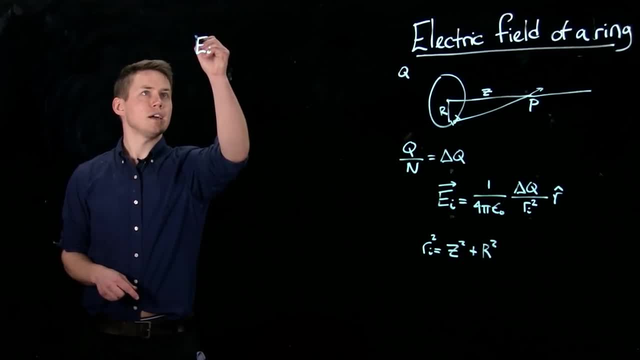 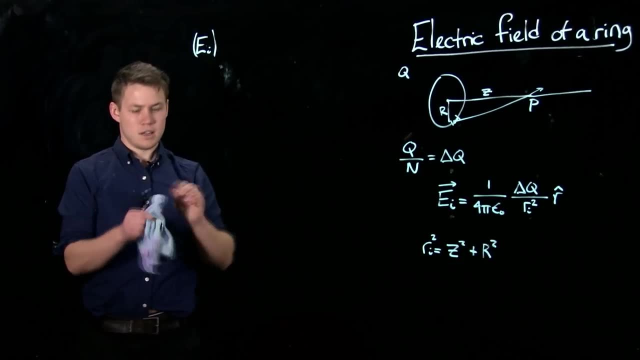 let's move over and do that just here. So, Ei, this is now a scalar and I'm going to use this notation. So this tells me. to make that a little bit clearer, this tells me: this is the electric field due to the i-th. 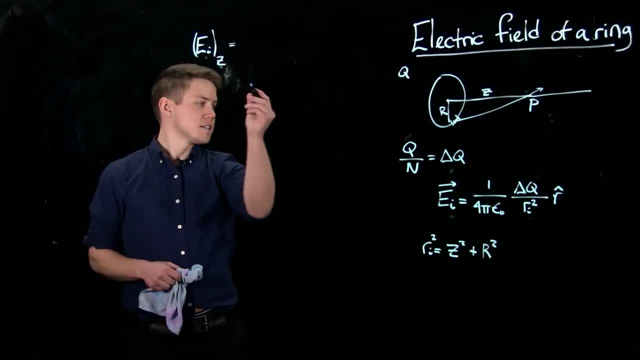 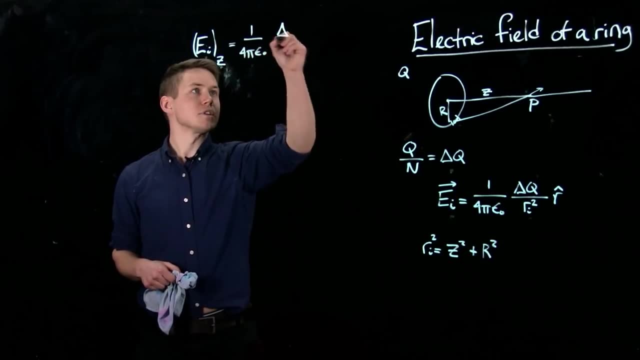 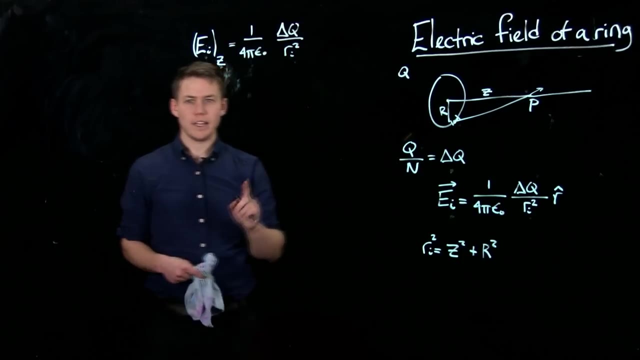 component along Z. Well, what is that? It's the magnitude of the electric field there: 4 pi epsilon naught. Then I have this delta Q and also the Ri squared. This remains the same, but now I need to take just the component of it in the Z-axis. 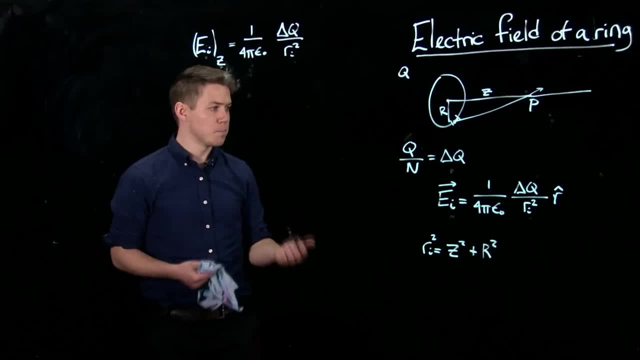 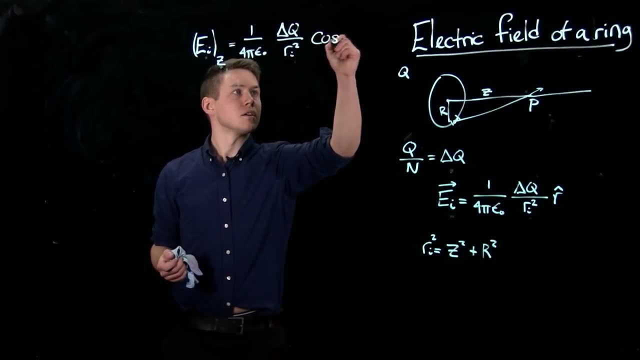 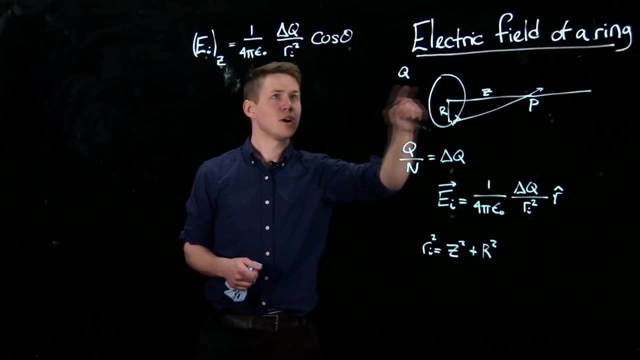 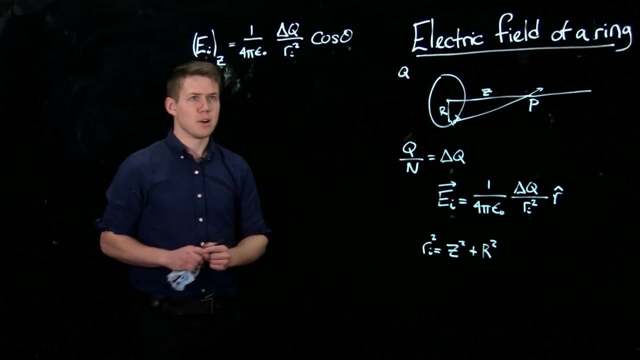 the Z-direction. So to get that I multiply by cos theta. So in particular, what this means is that if this angle is very small, ie if this radius goes to 0, then this term is going to go to 1, and all of the electric field is along the X- sorry, the Z- component. 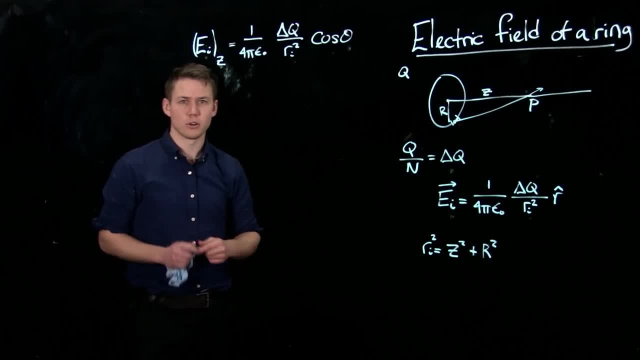 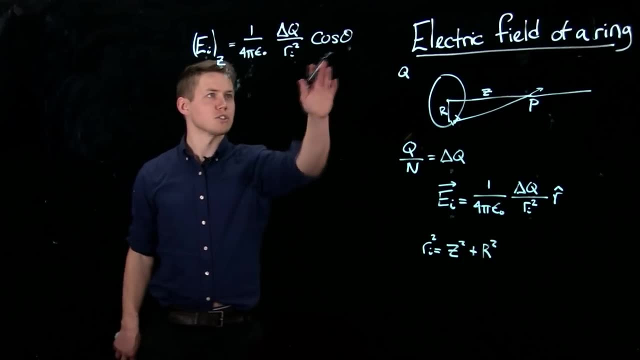 If you are a little bit confused about this, then ask a post on Moodle, of course, to try and clarify. I hope I've said enough there to make it clear. Ok, so what have I got? I've got this cos theta here. Well, I'd like to get rid of. 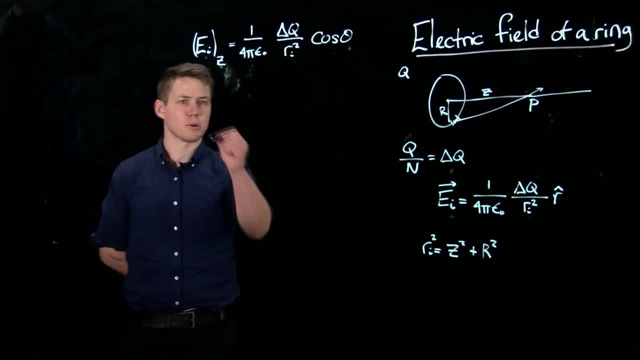 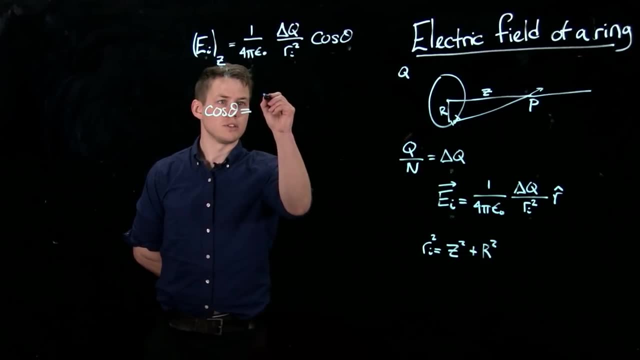 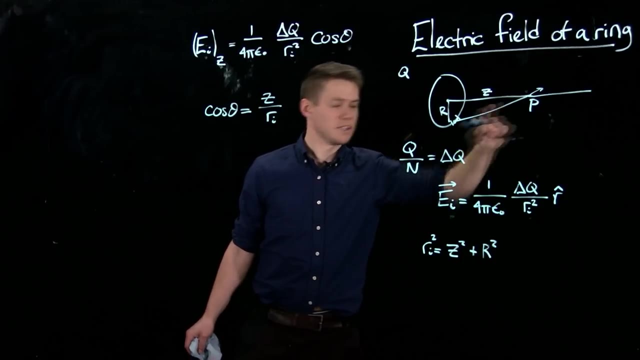 that because I can figure it out from all of the other lengths I have in the problem. So what is cos theta going to be? So cos theta is going to be equal to Z divided by Ri. So that's just this distance here divided by this distance. 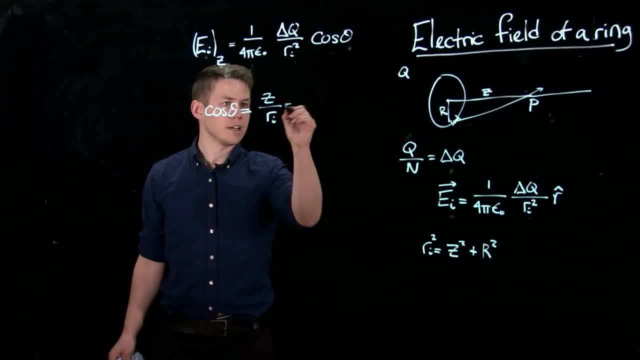 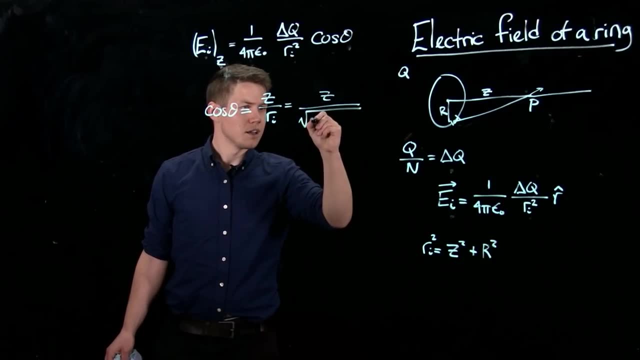 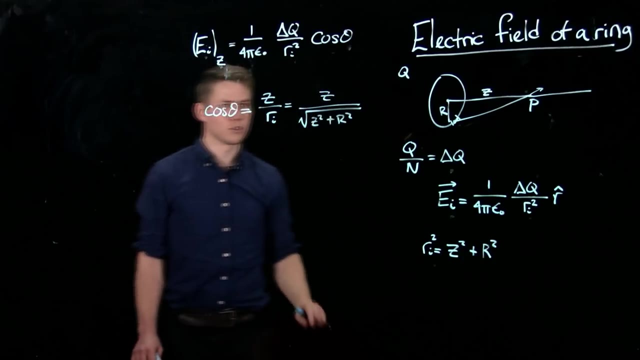 here. Well, of course, we already know what Ri is, so we can write this in a Z going to be equal to 1 over Z, over, sorry, Z squared plus R squared, taking that from this equation here and taking the square root, of course. Okay, so now I can. 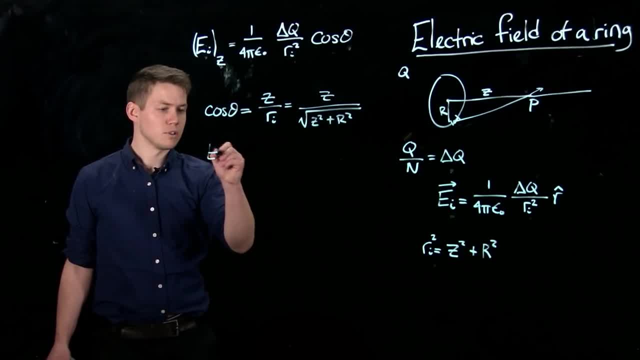 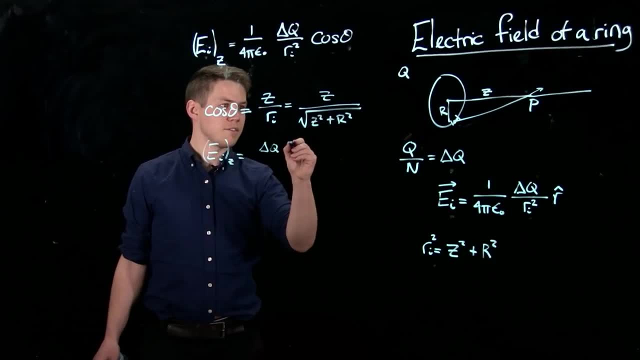 plug that in up here. so therefore EI along Z is equal to delta Q. I'm going to pick up a Z from here, and then I have 1 over R, 4 pi, epsilon naught. I have the ri squared here. Well, ri squared, as we said, was z squared plus. 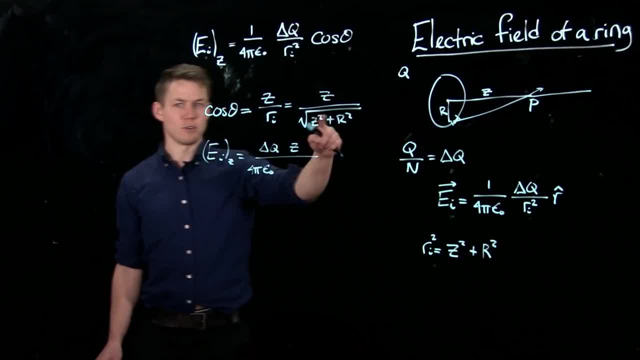 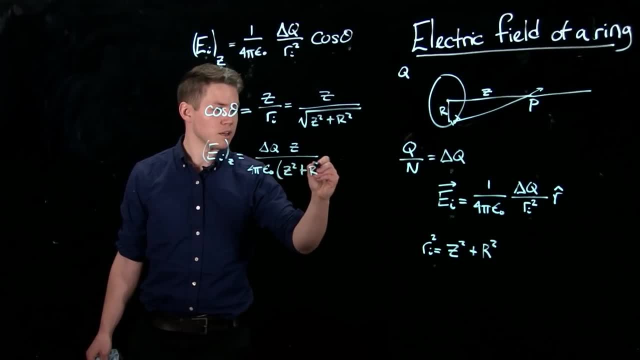 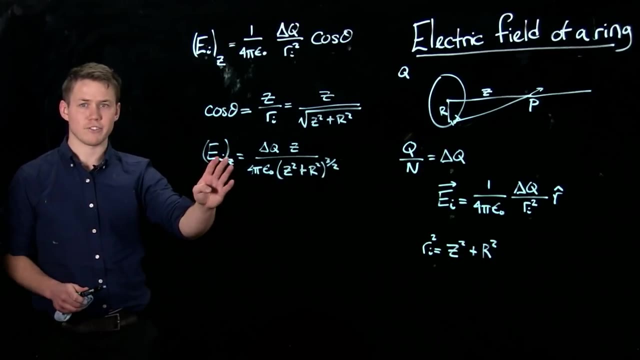 r squared, and then I'm going to multiply that by this square root right here, and so that's going to give me a factor of three halves, z squared plus r squared, all to the power of three halves. Okay, so what have I done so far? I've managed to figure out what the electric field is. 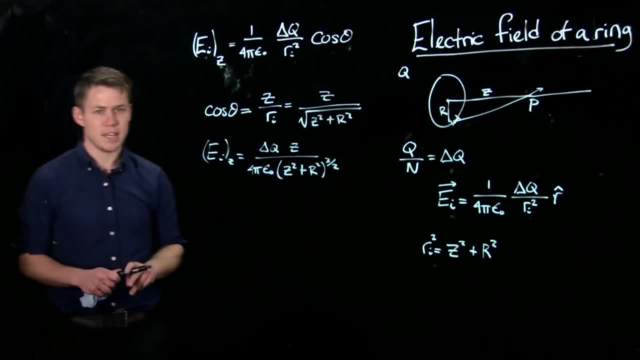 due to the i-th segment at p in the z direction. but what do I want? Well, of course I want the electric field from all of those n segments. How do I calculate that? Well, I can write it out here. 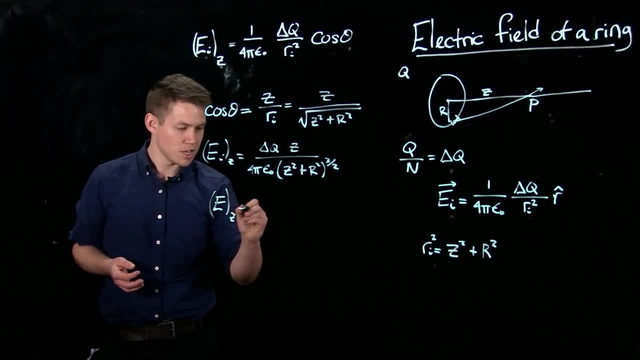 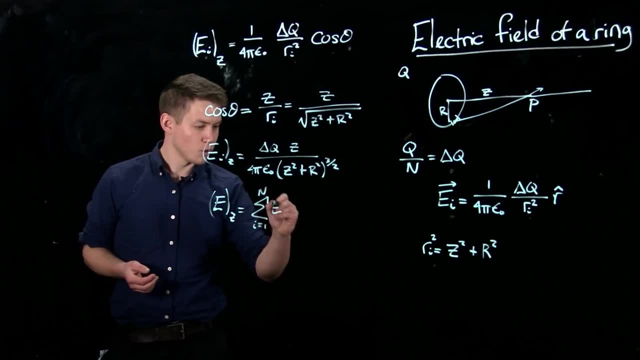 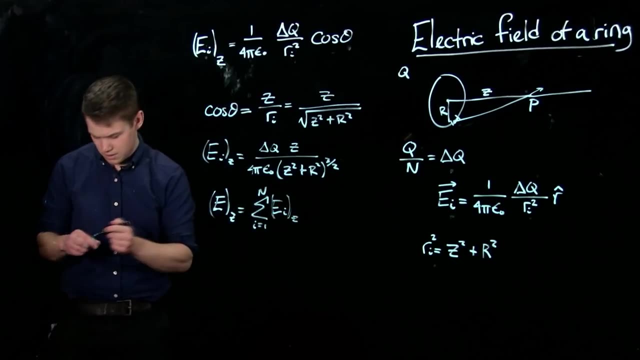 The electric field in general along. z is just the summation from. i equals one to n of all of these things that we've already calculated. The pen is slightly running out, Okay. well, this term is just given here. Now we notice something.